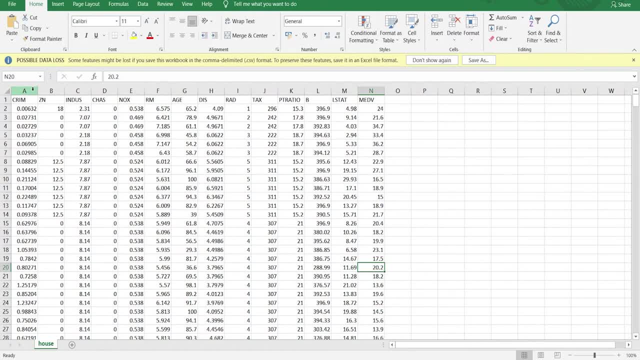 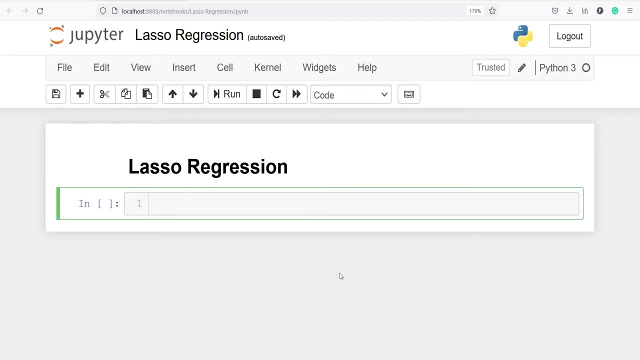 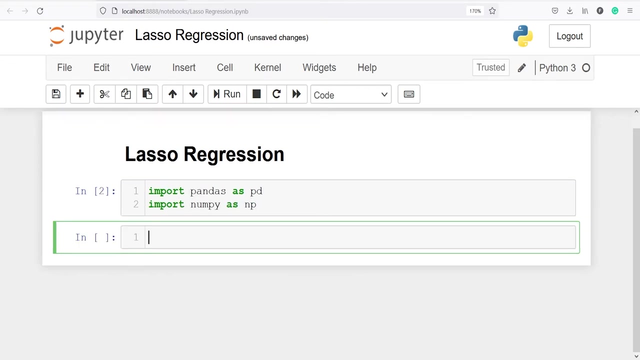 predict using our independent variables. All these rest of these variables are independent variables. Let's go to jupyter notebook and import this data set. Let's import pandas as pd, Import numpy as np. I'm going to make one variable df From pandas. I will call the method: read underscore csv. 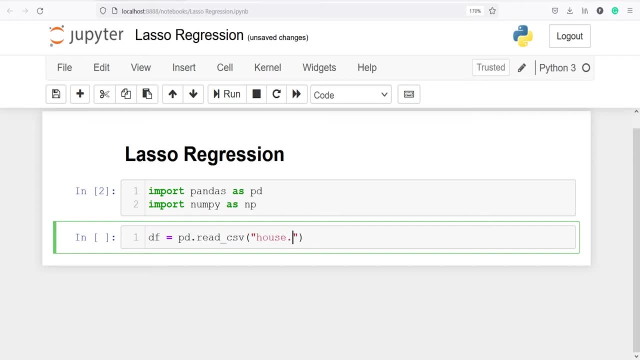 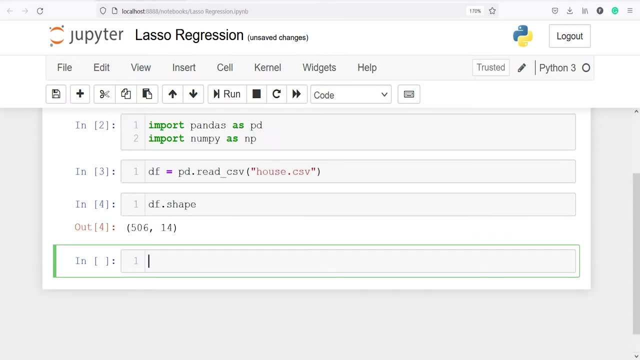 and inside this I will pass my csv file name: house dot csv. Let's explore our data set. First I will write df dot shape. In the output you will see we have 506 rows and 14 columns. Let's look at the head of our data set. We will use the method head: df dot head. 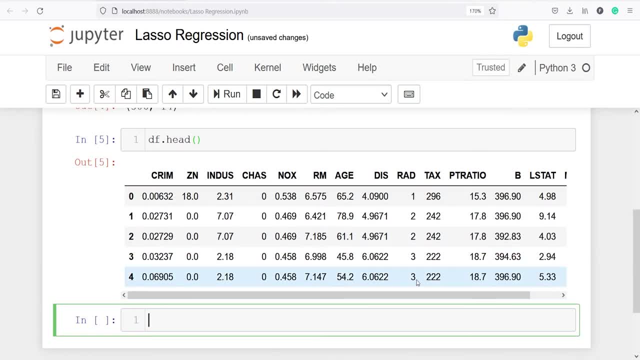 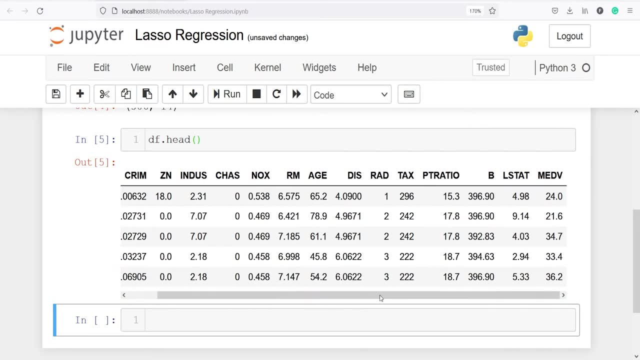 and this will give us the top five rows of our data frame. These are the top five rows and these are the column names, such as cr, im, zn, indus, chas and so on. madv is a target variable. We can also look at the bottom five rows of our data frame using the method tail. 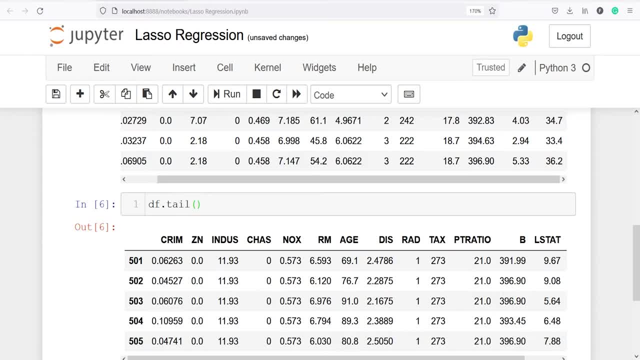 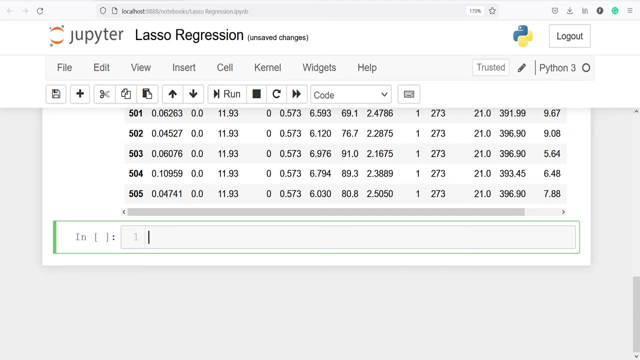 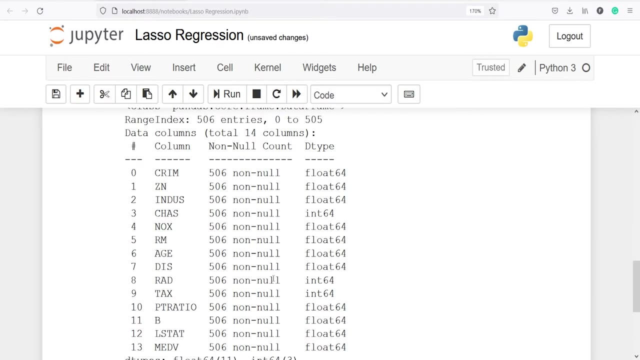 df dot tail. These are the bottom five rows of our data frame. We can also look at some other information using the method info. In the output you can see we have information such as the column names, non-null count and the data type. for each and every column We can also get the descriptive. 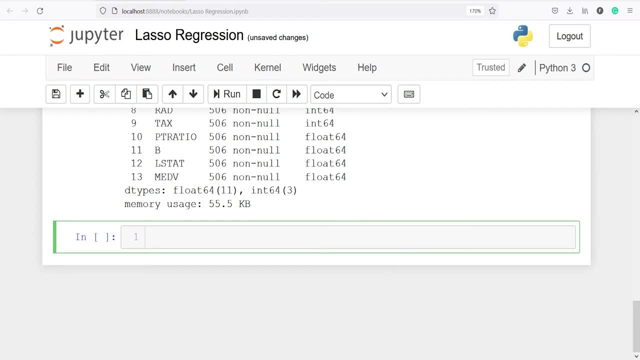 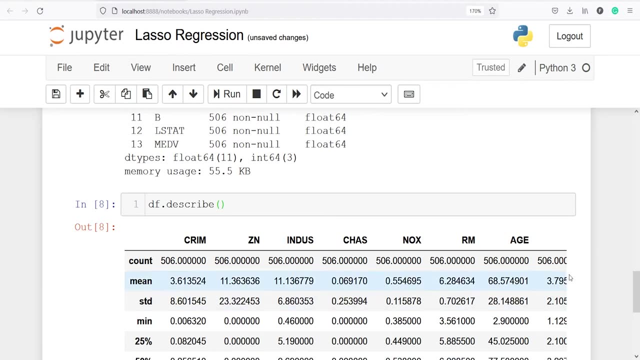 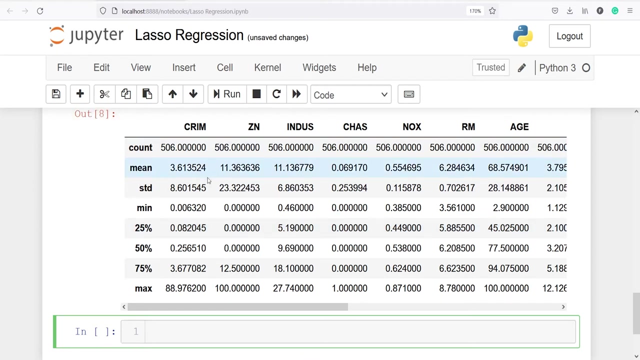 statistics for all the continuous variable and we will use the method describe. I will write dfdescribe In the output. you can see we got the descriptive statistics for all the continuous variables such as we have: count, mean, standard deviation minimum, 25%, 50%, 75%, maximum. 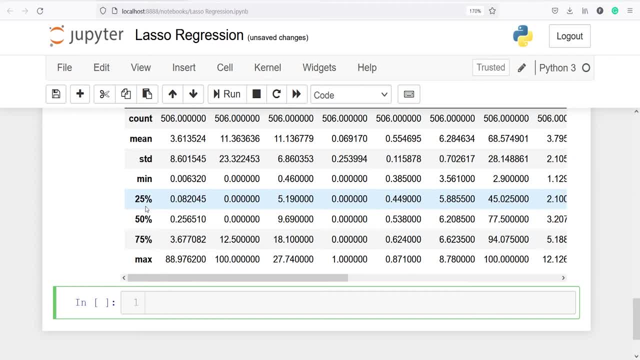 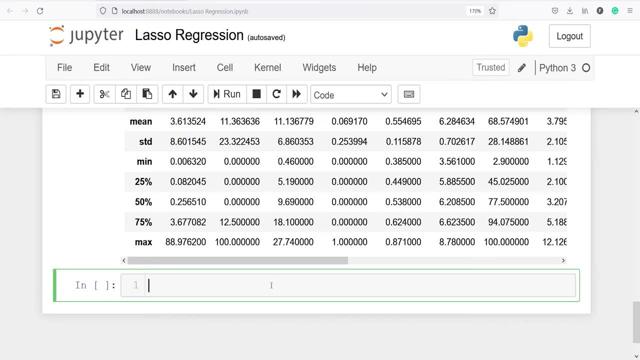 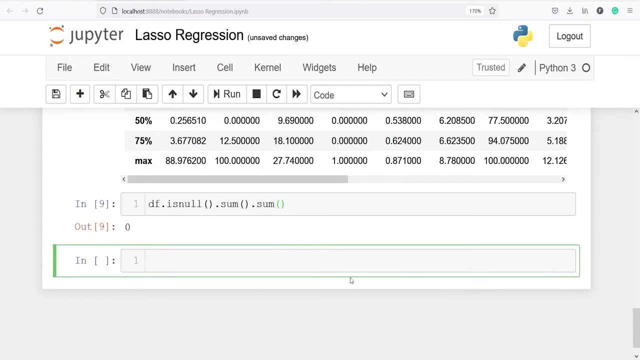 So these are the descriptive statistics here: 50% is medium, 25% is first quartile, 75% is the third quartile. Next, we can also check if there are any missing values present in our data set. We will write dfisNullsumsum, and here we got 0 because there are no missing values. 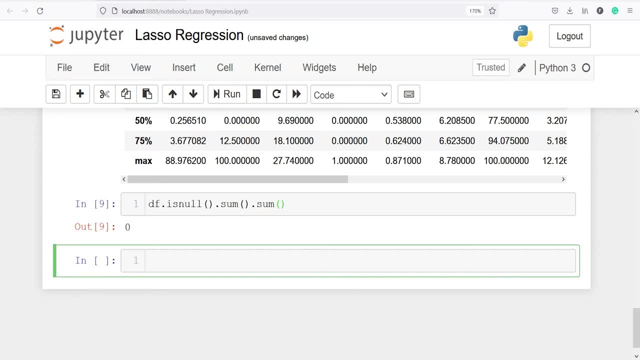 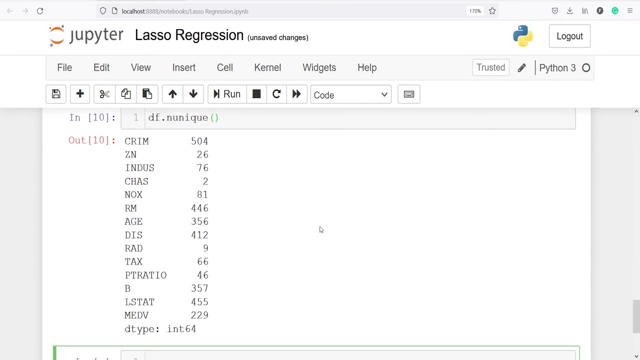 in our data frame. We can also look for unique values present in our columns, and we can do that using the method n unique. I will call dfnuniquesumsumsum, because that's where these things give us anything about values, and in the output we got the column names as well as the unique values that are. 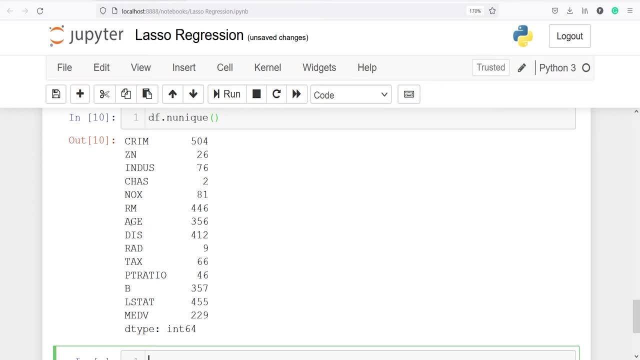 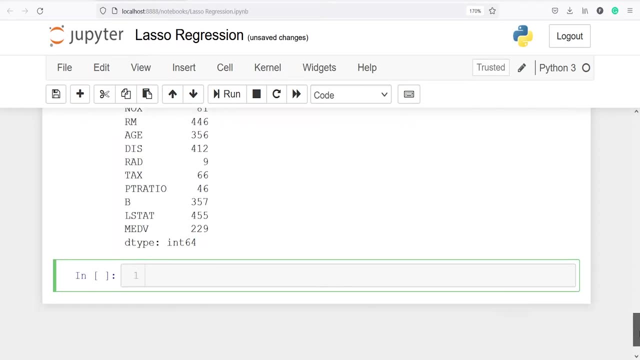 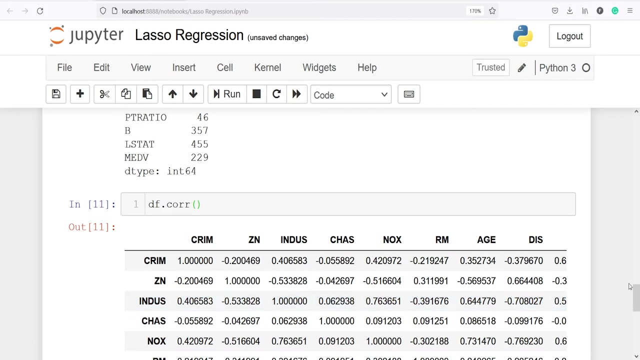 that are present in each and every column. for example, in column h there are total 356 unique values. in column b, here there are total 357 unique values, and so on. we can also get the correlation matrix. i will write df, dot, corr and in the output we got the correlation matrix. and here we can. 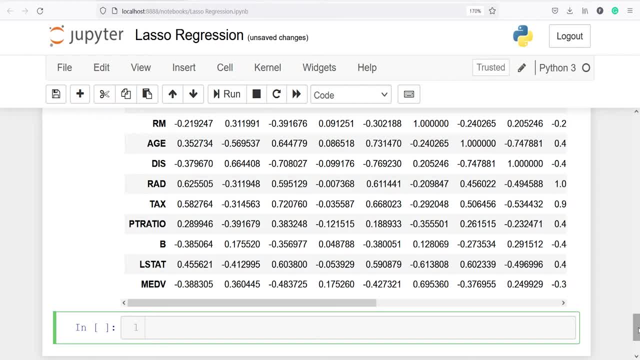 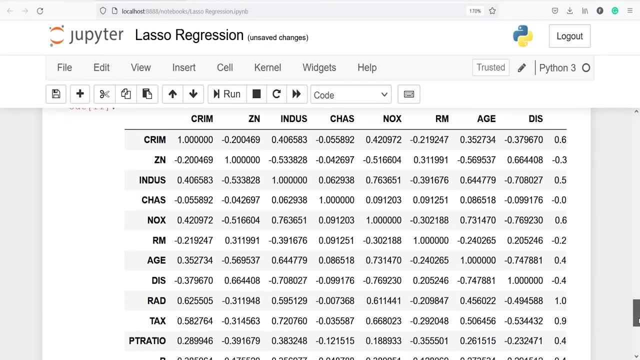 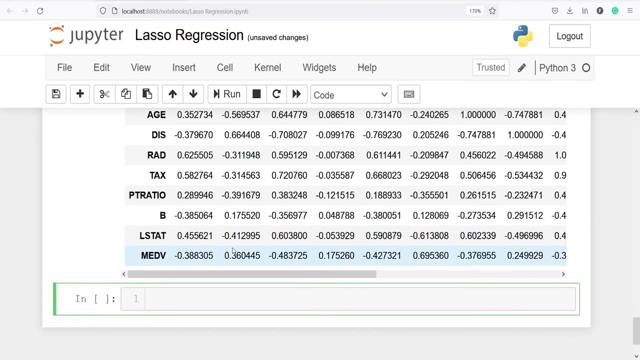 check the correlation between our independent and dependent variable here. our dependent variable is medv, that is the target variable, and we can check out the correlation with the independent variable here. for example, the correlation with the variable zn is 0.36, that is, 36 percent for other variables. 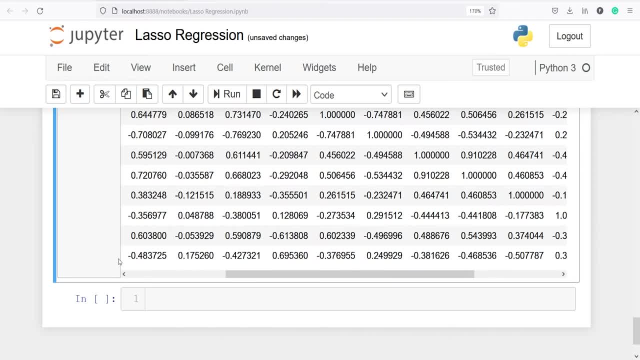 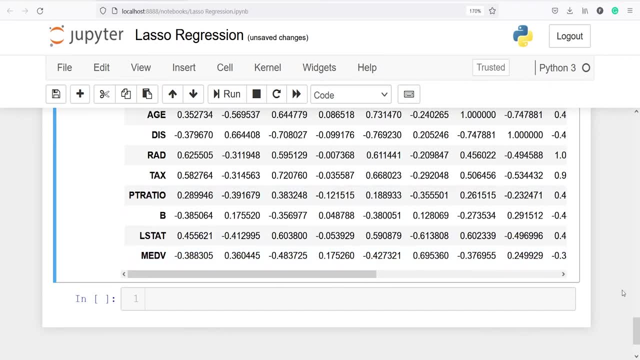 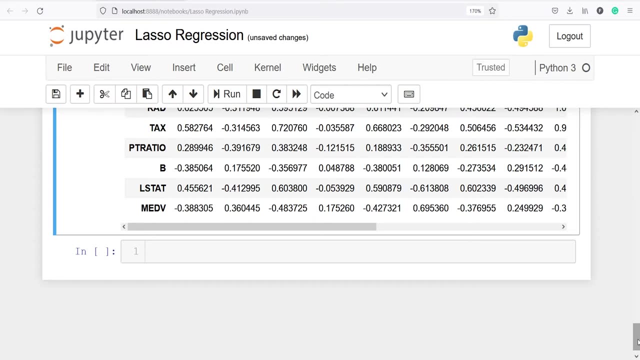 we have different collisions, such as minus 48 percent, 17 percent, minus 42 percent, 69 percent and so on. we can make a scatter plot to check the correlation and in a scatter plot we are going to include only few variables, because there are so many variables in this data frame. for that i need 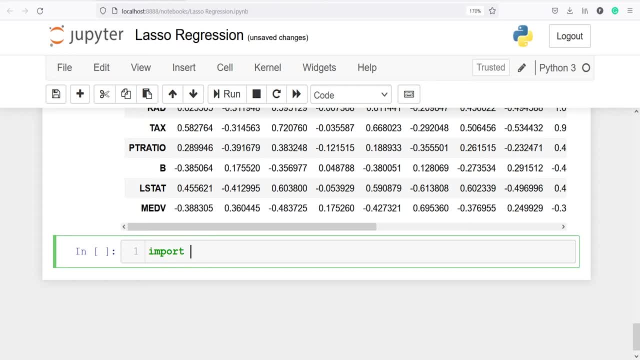 to import matplotlib. so i will import matplotlib, dot pyplot as plt from ml extend dot plotting. import scatterplot matrix. then i'll make one variable columns and this is going to be a list and i'm going to save some variables here on which we are going to make the scatter plot. for example, we will take variables: 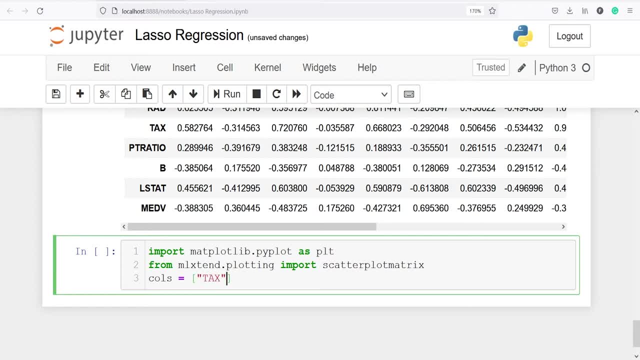 such as tax, then lst80, then rm and our target variable m, e, d, v. we will call this scatter plot matrix and inside this we will pass our data frame and we will subset it with the columns, because we want to get the scatter plot of these columns only and to get the values we will type dot values. 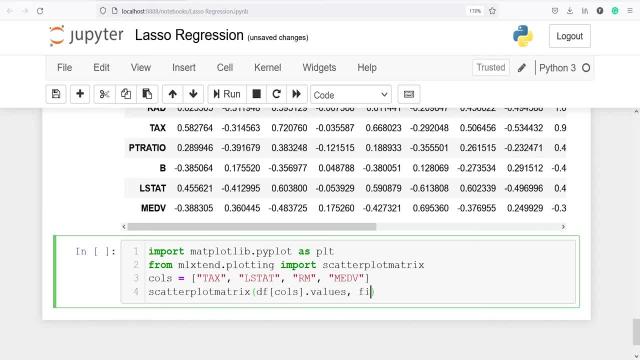 dot values. then i'll pass on parameter fix size. it is going to be 10 by 8. it is to adjust the size of our scatter plot. you can put any number here, depending on the requirement. the next parameter is names. so our names are going to. 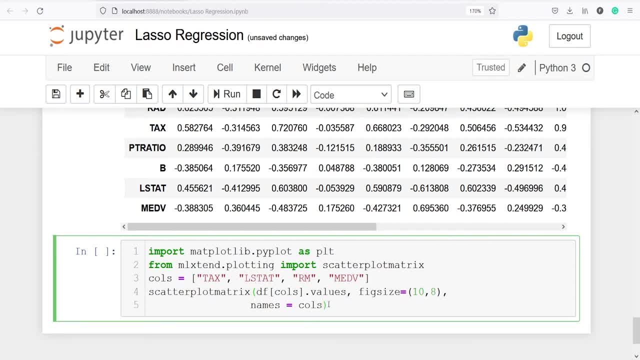 be column names, that is, the names that are saved in this list: cols. next parameter is alpha and we will take it as, let's say, 0.6. it is for the transparency of the color. then we will call plt dot- tight plot, tight layout and finally plt dot- show. let's execute our code. 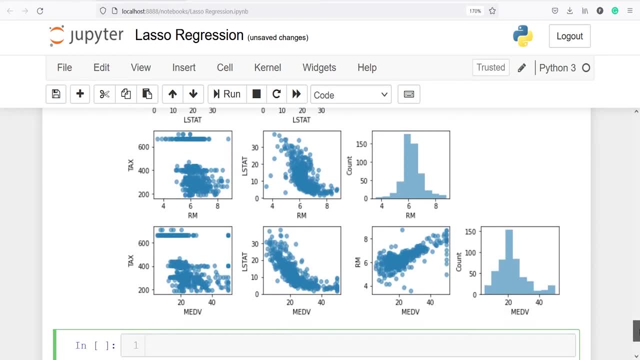 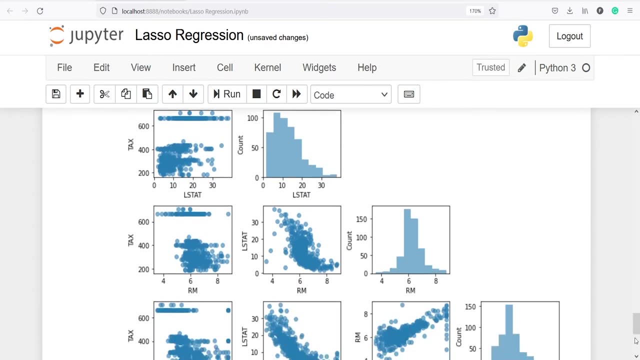 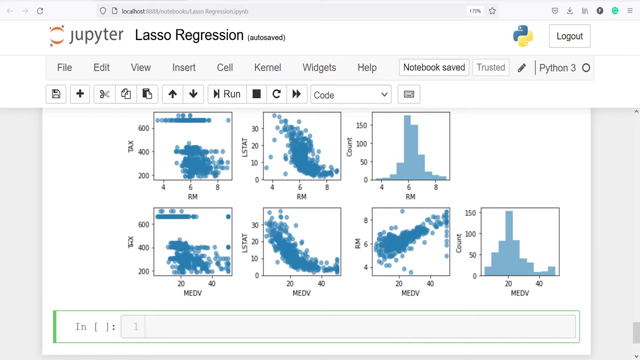 and here we got the scatter plot, here, or the scatter matrix. so we got this scatter matrix for few variables only, such as tx, lstat, rm and medv, and here we look at the correlation between: here you will see the correlation between tx and medv. there's no correlation, and here you will see the correlation between medv and. 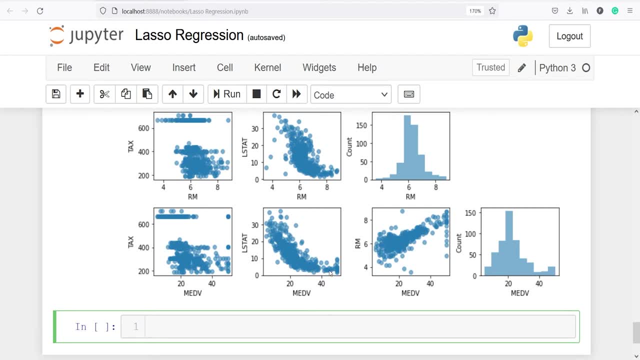 l start. it is negative coalition. it is going this. it is going in this direction. the left side- and if you look at the position between watches and mediv, you will see it has a good correlation. it is going in the same direction and here also you will see the 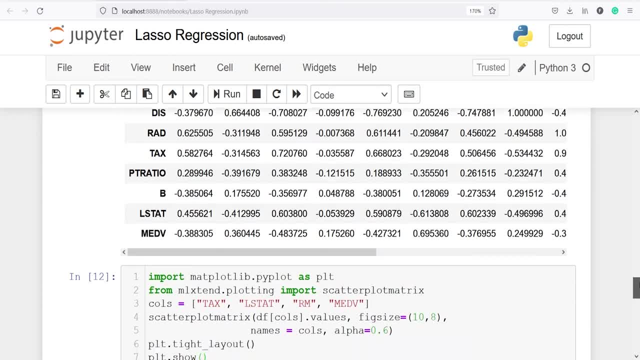 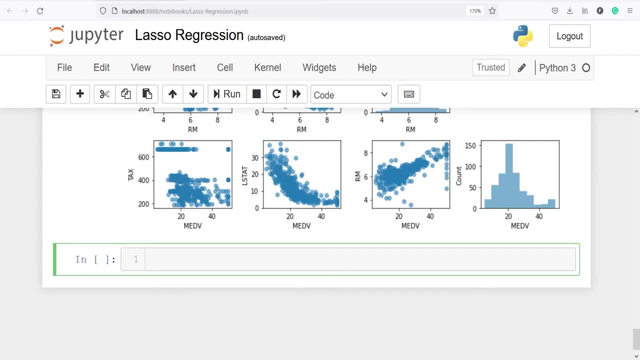 correlation between rm and medv is sixty nine percent. that is why in scatter plot we got a good plot here. next we will make the heat map for that. i will import from ml extend dot plotting, import heat map. so using this we are going to make heat map here. 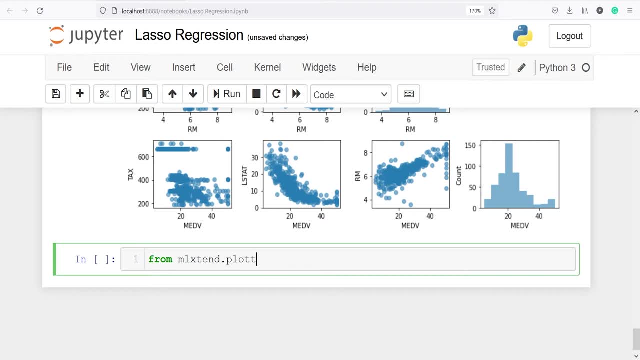 from ml extend dot plotting. i have to remove 1t import heat map. then i will make one variable, cm, and in this i will say the correlation coefficients of all the variables. and to get the correlation coefficients i will use the method curt-coef from the numpy. so i 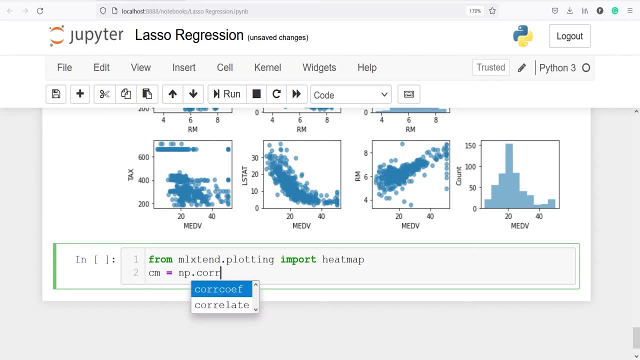 will call this numpy. from this i will call the method preparation coefficient and inside this i will pass columns, dot values, dot t. we want to get the coefficient, coefficient of columns present in this list, cols that these initial and initialmount. there i am going to move it just to. 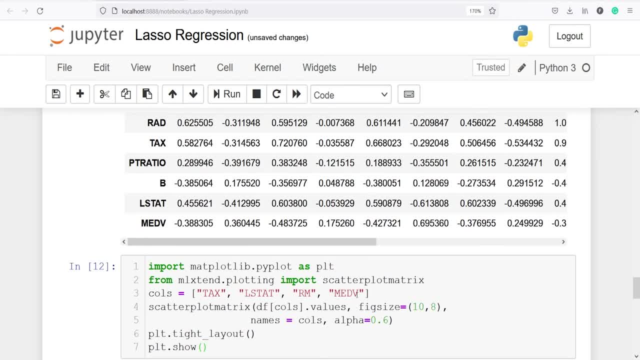 fails here that i will make hundred and hundred so you can see these numbers. no, this one is two, because there are only by lång- you need to весь it- the ratio of m seen around 0.2енс at the pivot. so is why we are passing this here. so we will get it for one, two, three and four. 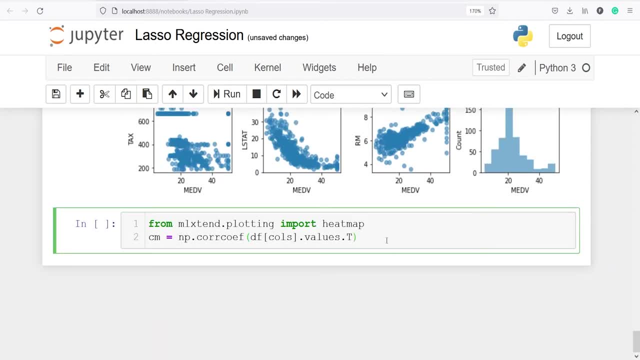 four variables only, and next I will make one more variable, HM, and in this I will save the heat map. so I will call heat map and inside this I will pass our variable CM, then row names: our row names are going to be same, that is columns and. 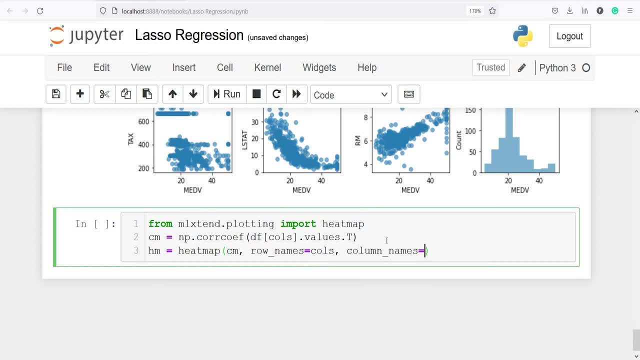 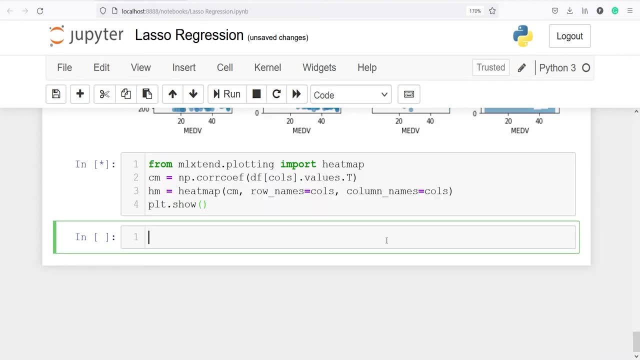 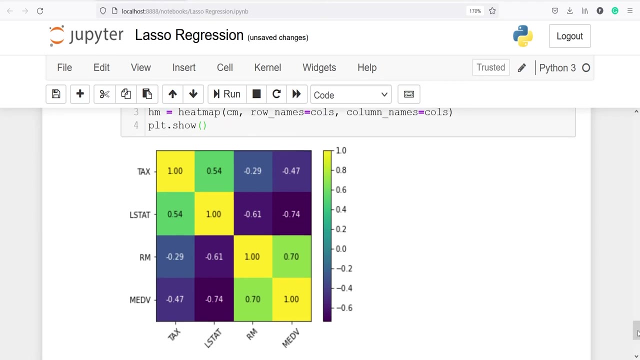 then column names. column names will also be same COLS columns. the next last is PLT dot show and here in the output you can see. we got the heat map here and this tells us the correlation between the independent and dependent variable or the target variable. here our target variable is MADV and we can check the. 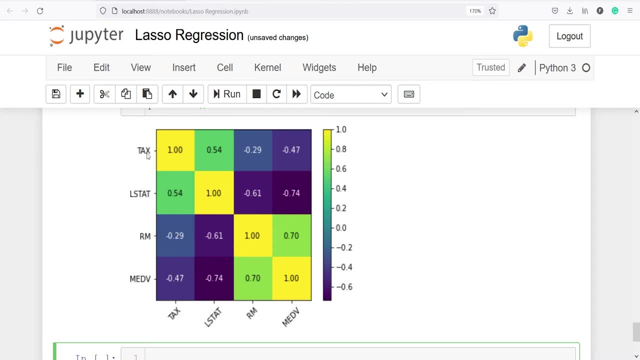 coalition with all the independent variables, that is, TAX, LSTAT, RM. so here you will see that the correlation between the independent and dependent variables is: between RM and MADV is 70%, between LSTAT and MADV is minus seven four percent and between tax and MADV is minus 47%. so next we will split our data. 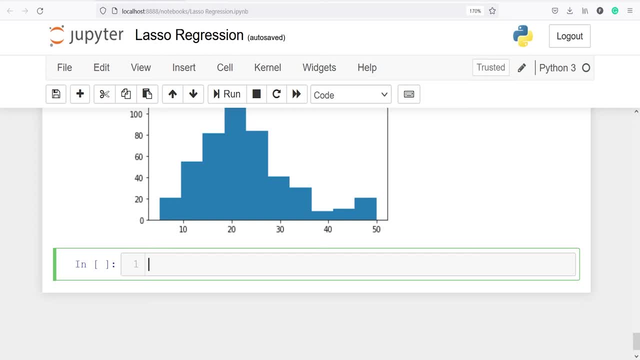 frame into X and Y. in extra will save all the independent variables and in why we will save our target variable, I'll make variable X. I'll call DF, ILO C if want all the rows. so I had type colon and I want all the column except the. 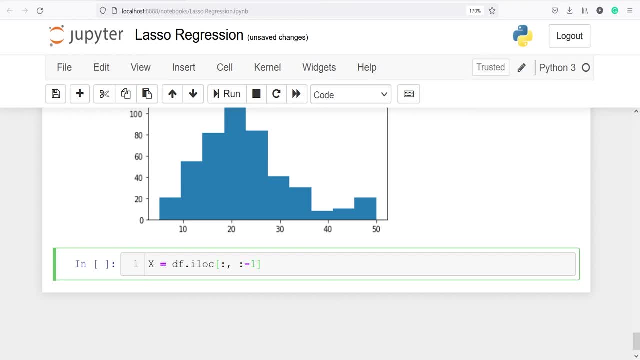 last column. so I will save all the about scroll and I will come here and I wanted to type colon и type colon minus one. and similarly for y, df, dot, iloc. i want all the rows and this time i just want the last column, that is the target column. so i will write minus one here. let's execute our code. 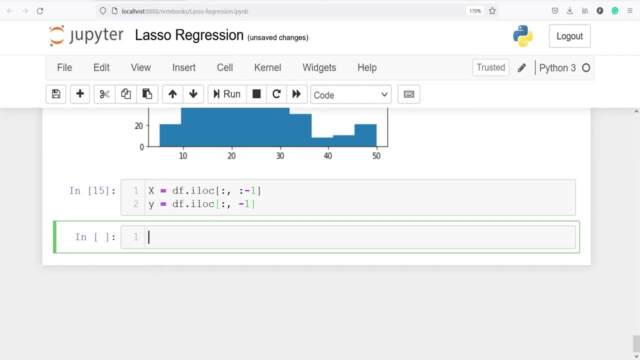 next i am going to split the data set x and y into train and test. for that i will import from sklearn one dot model selection: import train test split. now i will make x train, x test, y train and y test. then i will call train test split. inside this i will pass our data frame x and 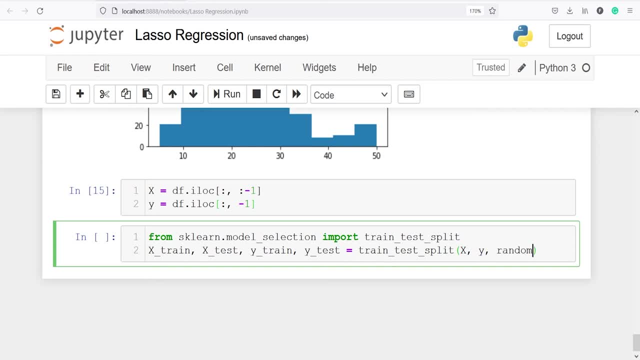 y and i will pass one more parameter, random, under score state. you can give any value. here let's say zero, but if you want your result to be same as mine, then you also have to put zero. here let's execute our code. we can check the shape of our x. 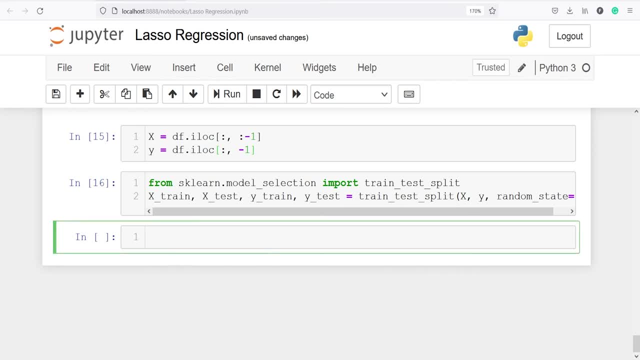 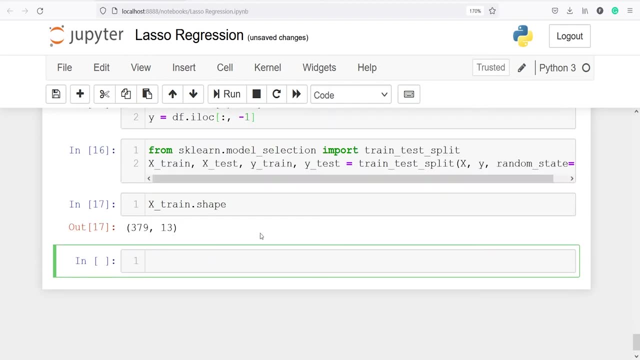 train and y train. so i will write x train dot shape. so there are total 379 rows and 13 columns. then we will also check for y train dot shape and here we have 379 rows. we only have target variable here. next we are going to import the lasso. 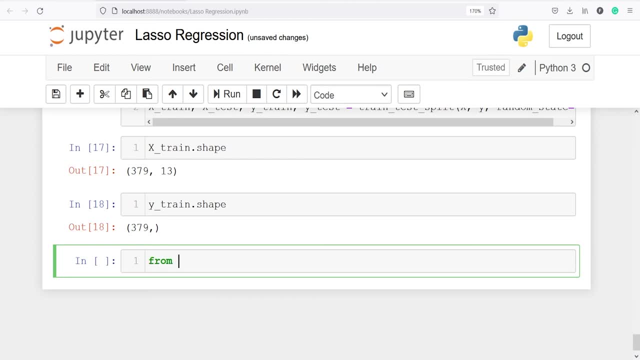 regression. so i will write from sklearn dot linear model import lasso. now i'm going to make the object of this lasso regression. let's say i will write lasso and then i will call this lasso here and i will pass one hyper parameter: alpha. 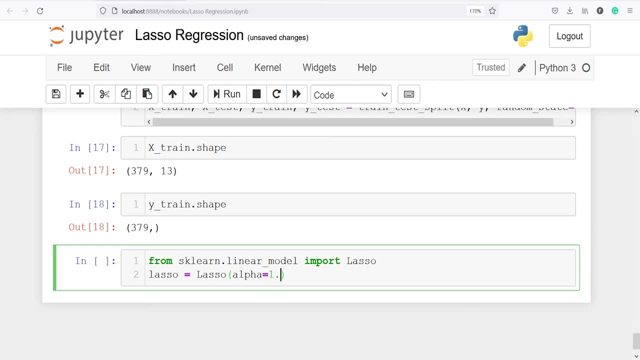 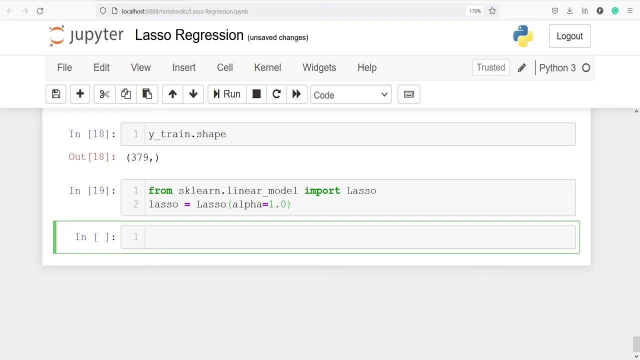 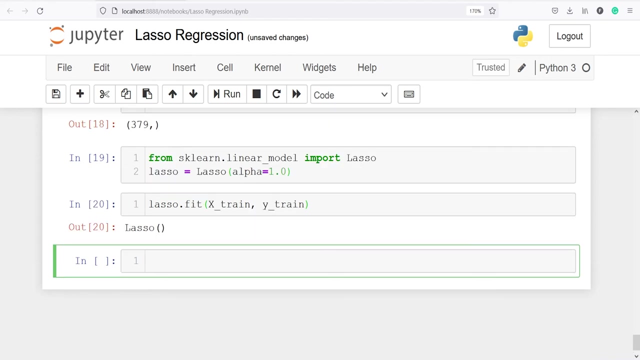 and its value is going to be, let's say, 1.0. let's execute our code. next, i'm going to fit it on our x train and y train, so i will call lasso dot fit and i will pass x train and y train and let's execute our code. so we have fit the model, the lasso regression model, on our x train. 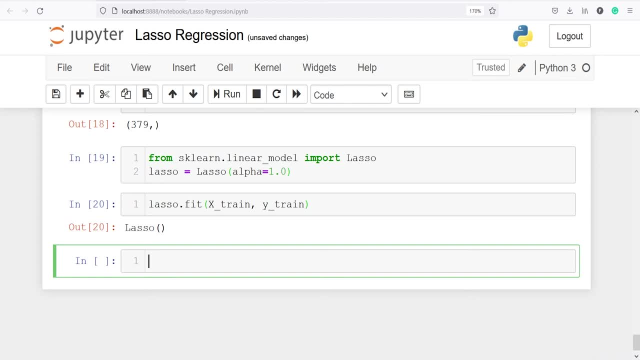 and y train. next we will make the prediction and save it in a new variable. i'll make one variable, y underscore pred, and in this i will save the predictions. for that i will call the object lasso and from this i will call the method predict and inside this i will pass x test because we want to. 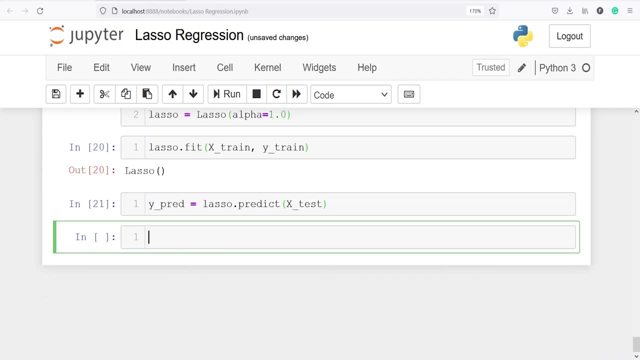 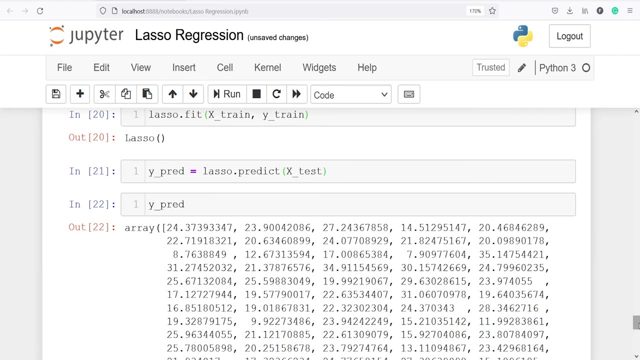 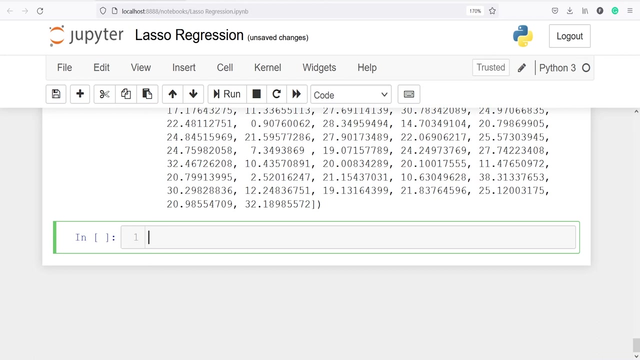 make predictions on x test. let's look at some of the predictions. I will call this variable yPred here. in the output you can see these are the predictions. these are the predicted median values of the house. next we will print the slope and intercept. let's first print slope. print slope percentage- dot 2f. 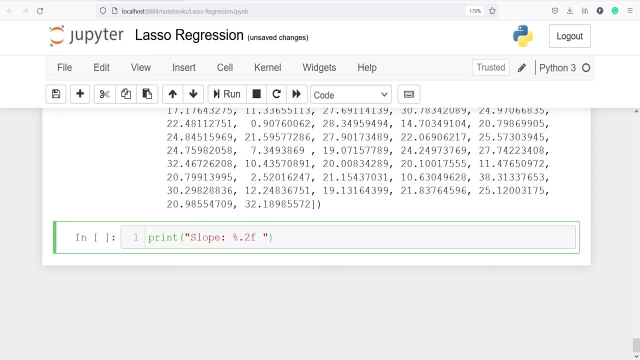 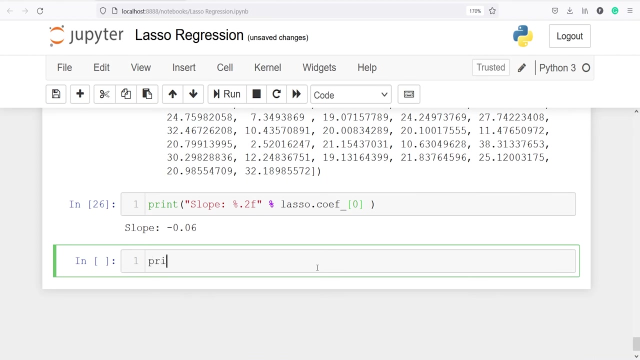 because I want to print this in 2 decimals only. that is why 2f here, then percentage less so, and the slope is present in this. coefficient index number is 0. let's execute our code. our slope is negative, 0.06. let's also print the intercept: print, intercept. 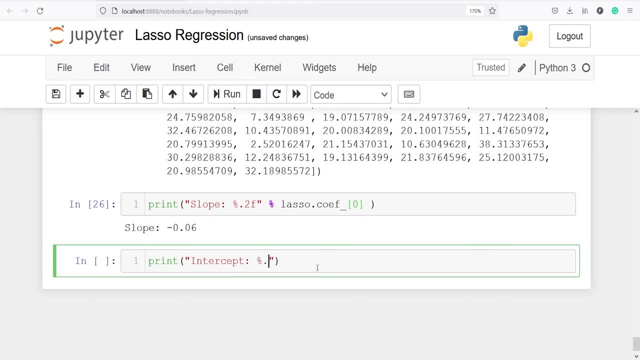 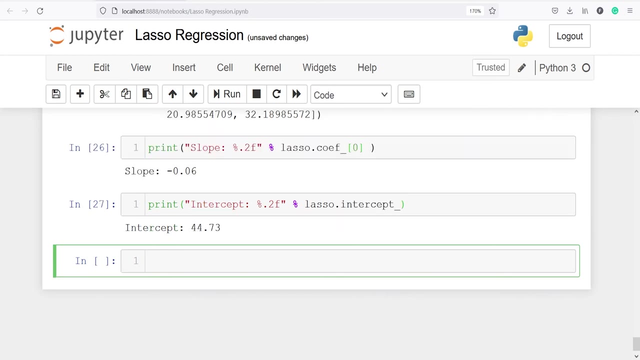 and this. this is also going to be in 2 decimals, so I will write 2f here. percentage less so dot intercept. let's execute our code. so our intercept is 44.73. now we are going to evaluate our model. we have fit the model. we have also made predictions. now it's time to evaluate the. 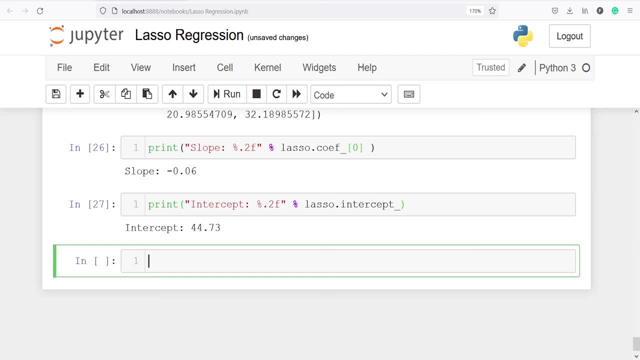 performance of our model and for linear regression or any type of linear regression we have to do linear regression like lasso, reach and etc. we use the matrix such as the msc or rmsc. so from sklearn dot matrix we will import mean square error. now we will call this mean. 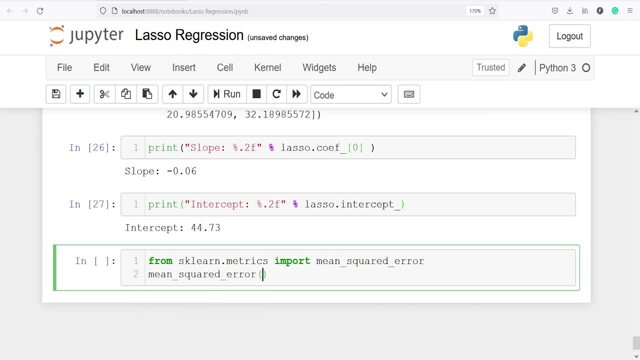 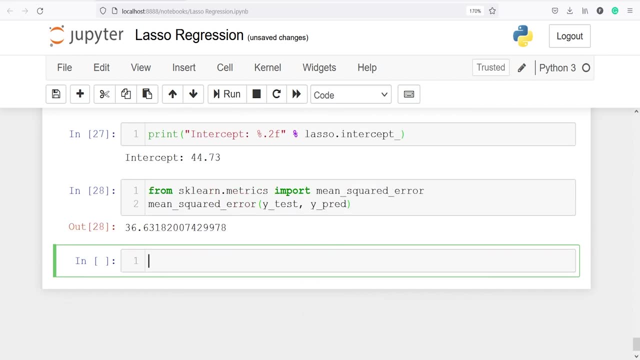 square error and I will pass ytest and yPred. let's execute our code and you can see that the msc is 36. we can also get the rmsc, and rmsc is nothing but the square root of this msc. and to get the square root first, we will call number and.